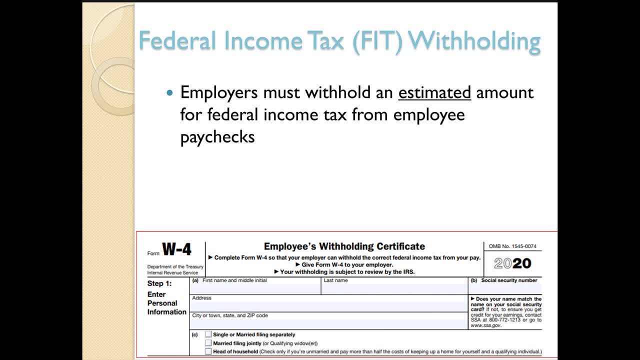 federal income tax withholding, FIT withholding. So employers must withhold an estimated amount for federal income tax withholding. So employers must withhold an estimated amount for federal income tax from each employee's paychecks. It's an estimated amount. So at the end of the year 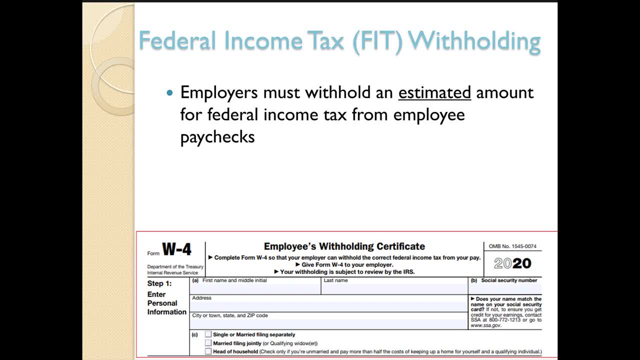 the employee will either have to pay a little bit extra, or maybe a lot extra, or they might get a refund back from the IRS. So how do we find out how much to withhold from an employee's paycheck? Well, first we need a form W-4.. This is filled out by the employee and is 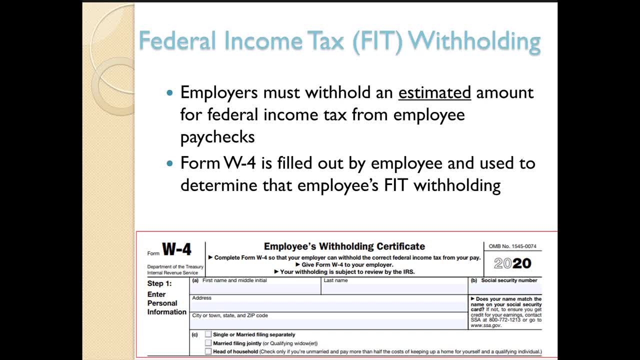 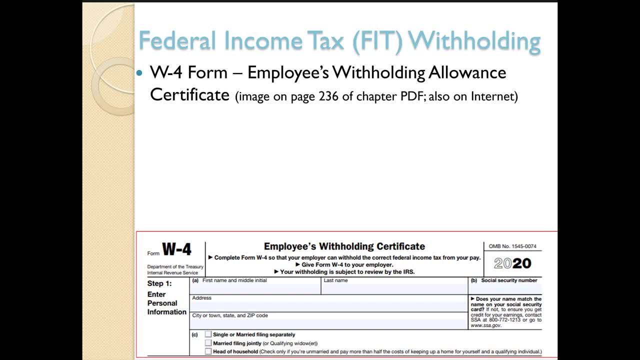 used to determine that employee's federal income tax withholding. So form W-4 stands for Employee's Withholding Allowance Certificate. No one calls it that. Everyone just calls it a W-4.. It's also on page 236 of your chapter PDF and you can also find the most current copy on the. 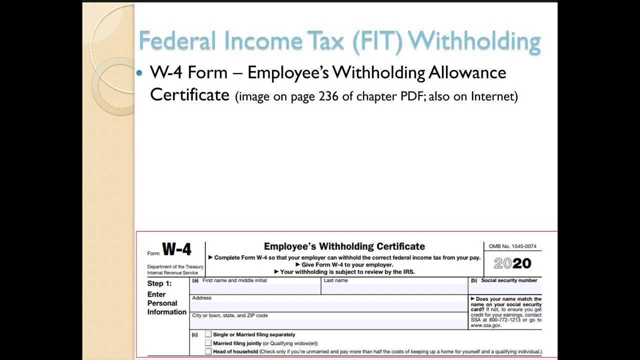 internet. So we've got an image at the bottom of the screen showing you the 2020 W-4.. So this form is completed by the employee when the employee is hired. The key components are the total number of allowances. Generally, an employee gets one allowance for themselves. 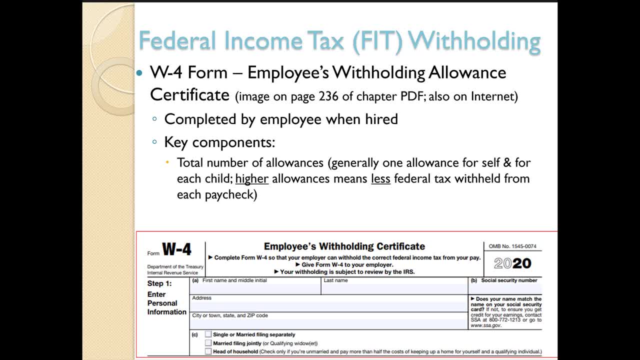 and one for each child. The higher the number of allowances, the less federal income tax is withheld from their paycheck. Now, some people really hate to have money withheld from their paycheck, so they like to have higher allowances. Now, if the allowances 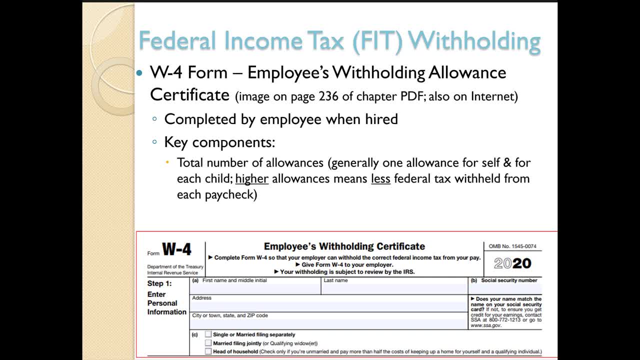 are too high. that means not enough federal income tax was withheld from their paycheck, which would mean that they have to pay a lot at the end of the year when they do their taxes. Another key component for calculating the federal income tax is the employee's marital. 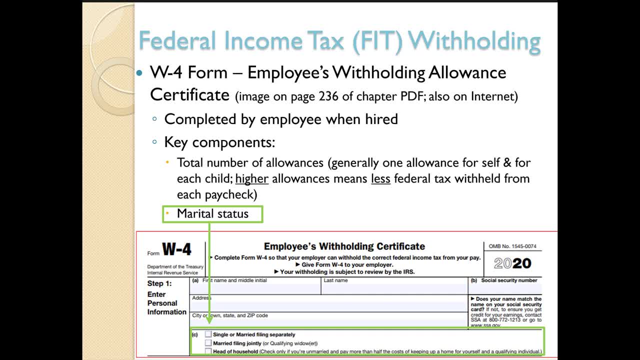 status. Now, when calculating the total number of allowances, I have some advice for you when you work in payroll- Now, when I was working in payroll- people would often ask the payroll folks: well, what should our allowances be? You should show them how to calculate it. 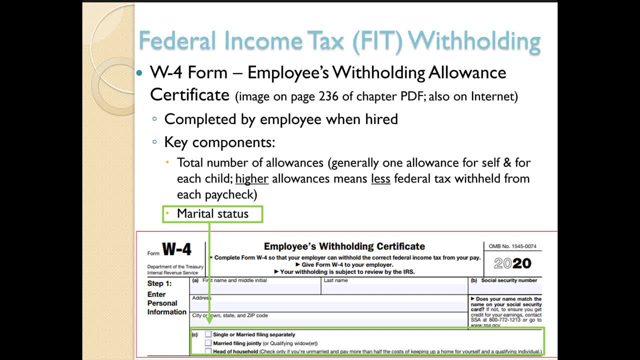 and it's just an estimate. There is no hard and fast rule for it. However, if you tell them what to have, they're not going to be able to calculate the total number of allowances. They're not going to be able to calculate the total number of allowances They're going. 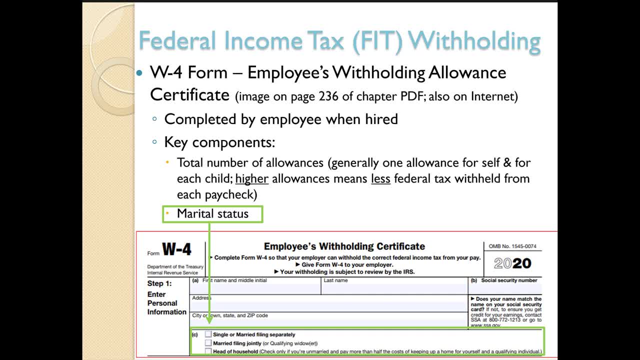 to be able to calculate the total number of allowances They're going to have to pay the actual amount of allowances. So if you tell them what to have, what to use for a number of allowances, oftentimes they will be unhappy at the end of the year with their refund or the amount they had to. 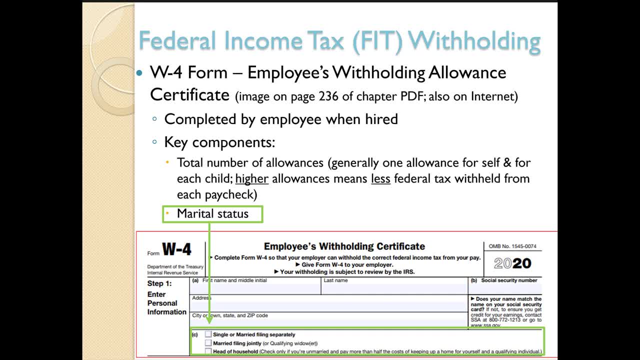 pay, so they'll come back and blame you. So don't give advice about how much their allowances should be. but you can help them fill out the W-4 and explain to them how it works, especially explain to them that the higher number of allowances, the less federal income. 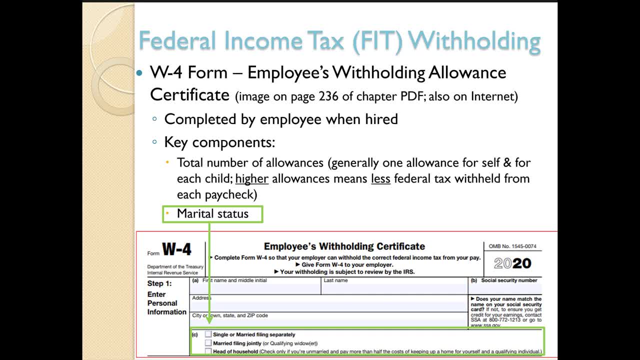 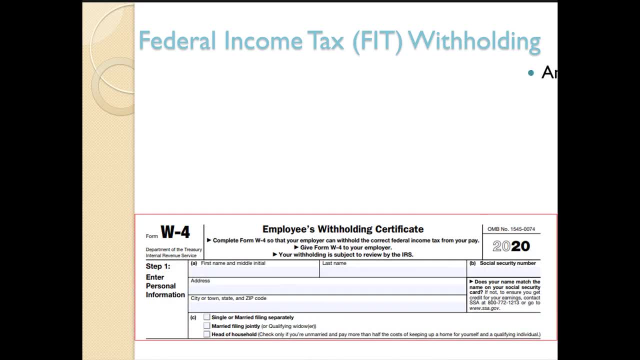 tax will be held from each paycheck, which would mean their paychecks would be higher. but if it's not that much, then you're going to have to pay a lot of allowances. So if not enough is taken out, they're going to owe a lot at the end of the year. 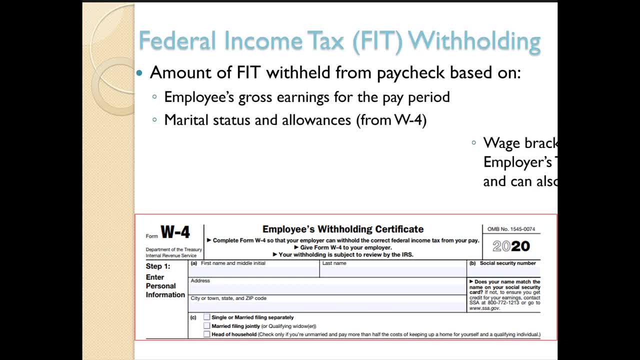 So the amount that we're going to withhold from an employee's paychecks for federal income tax depends on a few things. It depends on the employee's gross earnings for their pay period. Remember, gross earnings just means their gross pay, which means their pay before. 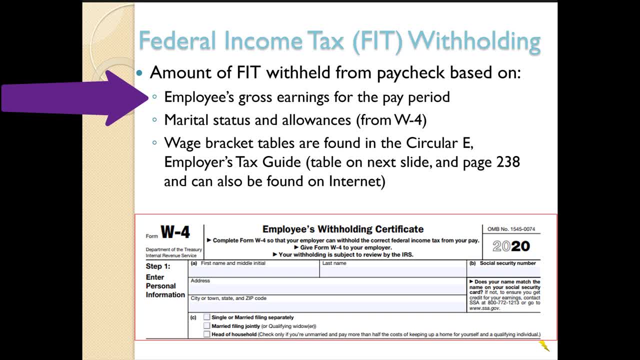 any deductions. So federal income tax is based on their pay before any deductions. It also depends on their marital status and their number of allowances, And again we get that from the Form W-4.. And then so we take the employee's gross earnings for the pay period, we take their 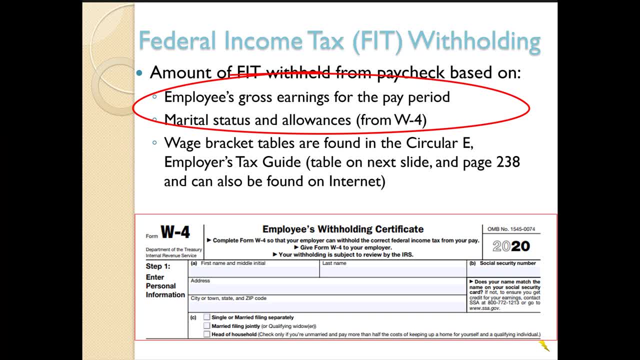 marital status and their allowances, and we look up this information on something called a wage bracket table, which we will do on the next couple of slides. So we're going to go over some examples And technically they're found on the internet in circular E- Employer's Tax Guide, But we're going to get some practice on these. 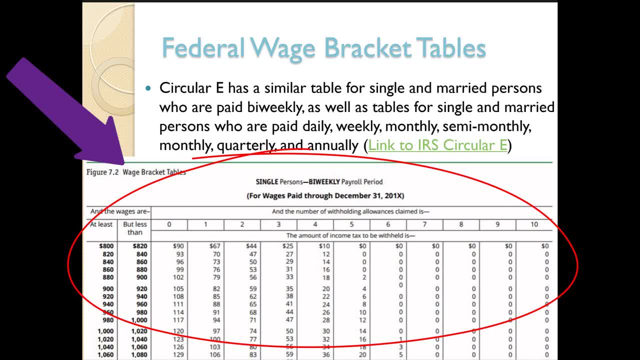 So this is what a federal wage bracket table looks like. So on the left, where it says: and the wages are, we would look up the employee's gross wages for that pay period And then we go across the line to find out how or and look up how many wages are included in. the pay period. So we're going to go across the line to find out how, or and look up how many wages are included in the pay period. So we're going to go across the line to find out how, or and look up how many. 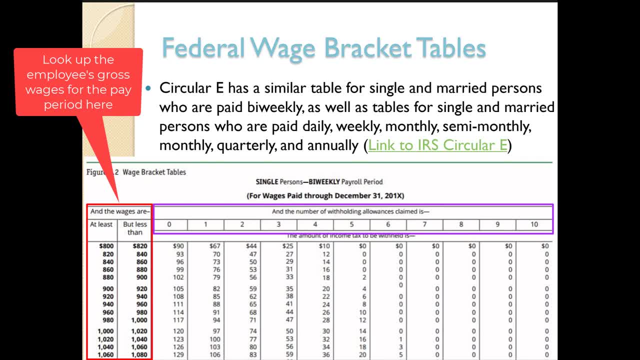 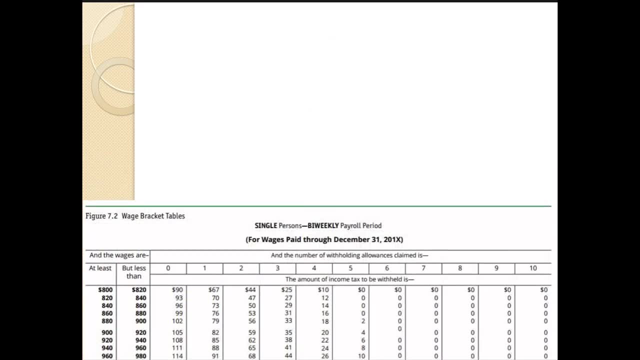 allowances they have, and then that amount is the amount we would withhold from their paycheck for that paycheck for federal income tax. So let's do one, or a couple, for practice. So we're going to calculate this employee's federal income tax withholding. So this employee is single, so we need to make sure that the wage bracket table we use is for single. 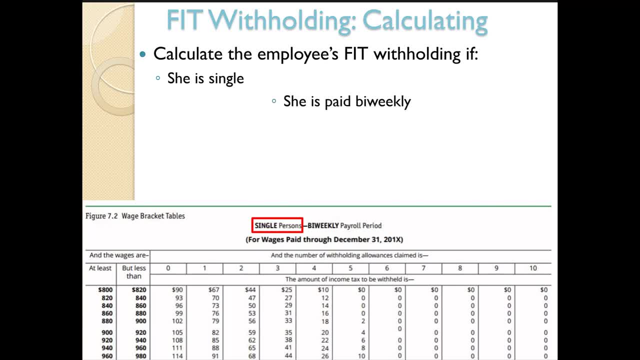 people. She's paid bi-weekly. so again you need to find the wage bracket table. that's for bi-weekly payroll periods And she claims one allowance. so we had to find the column for one allowance. And then we need to know her gross wages. So her gross wages for this paycheck are $830.. 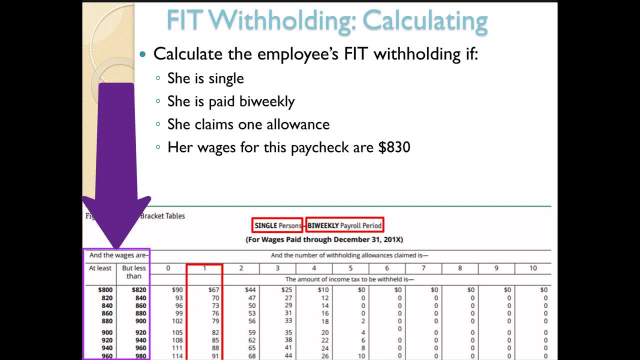 So in the left column, under the and the wages are, at least we use the $820 to $840 range. So now we can see that we're going to withhold $70 from this paycheck for this employee. and then let's take a look at the payroll bracket table. 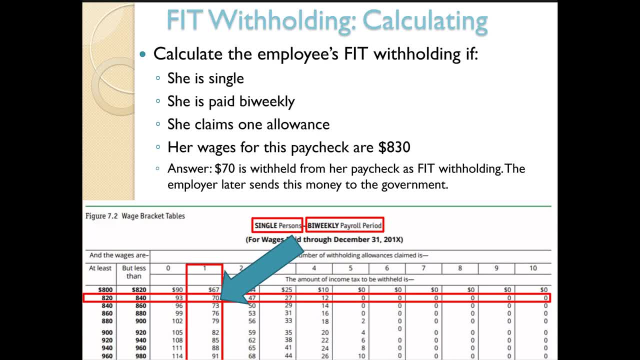 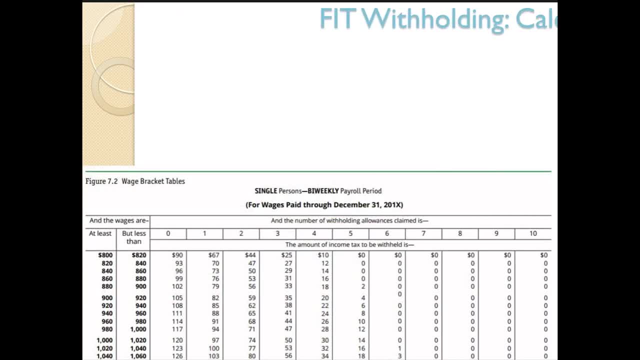 later on the payroll, people will give this money to the government, so let's do another one. we're going to calculate the employees federal income tax withholding. if she's single, so same table. she's paid bi-weekly, so again the same table. this time this employee claims two allowances and then we need their gross wages, her wages for. 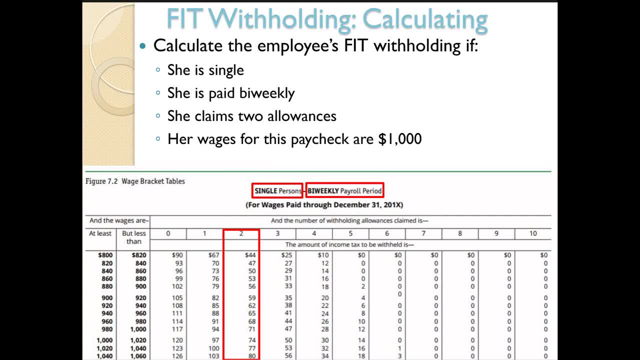 this paycheck are $1,000, so go ahead and calculate that before I show you the answer. the row you need to use on this one is a little bit tricky. notice: the row above the one that I selected says at least 980, but less than 1000. 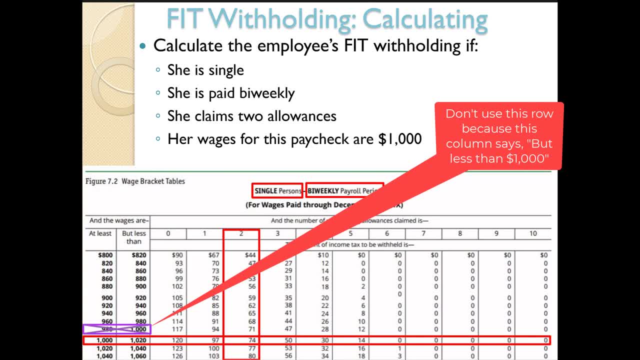 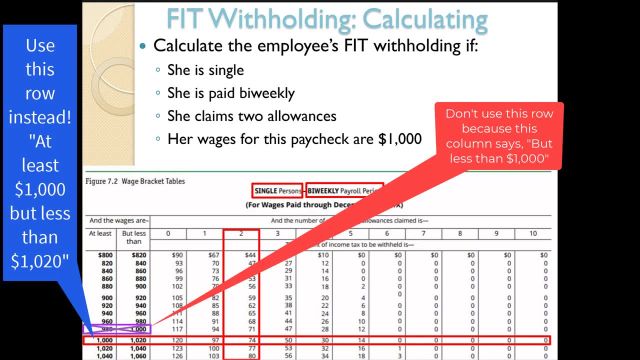 so 1000 is not less than 1000. so we can't use the row that says 980 to 1000. we have to use the row that says at least 1000 but less than 1020. so for this person, the amount federal income tax. 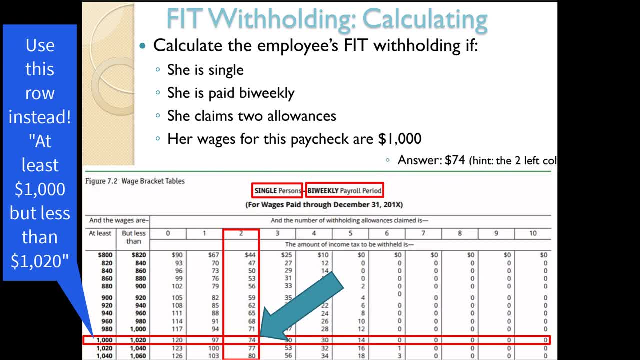 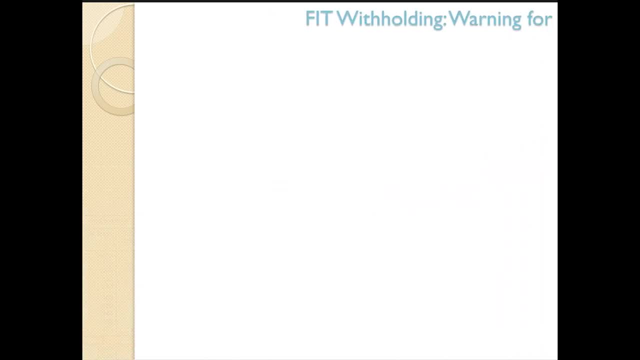 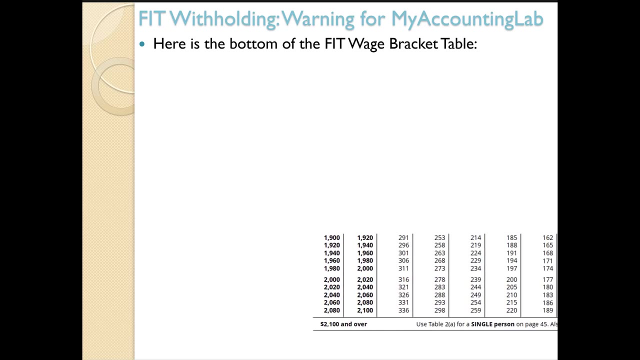 we're going to withhold is $74. so really be careful about reading those two columns on the left. they say at least and but less than. I've got a warning for you about looking up federal income tax withholding in my accounting lab. so here's the bottom of the federal income tax wage bracket table, if an 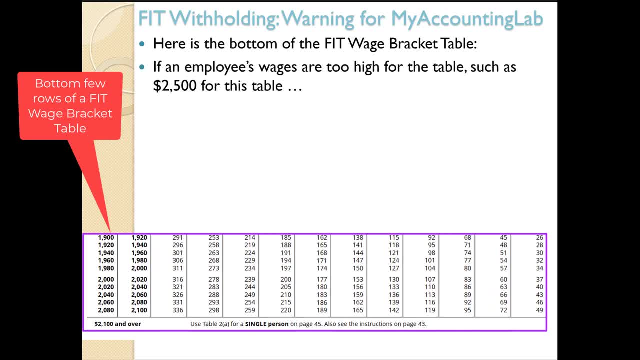 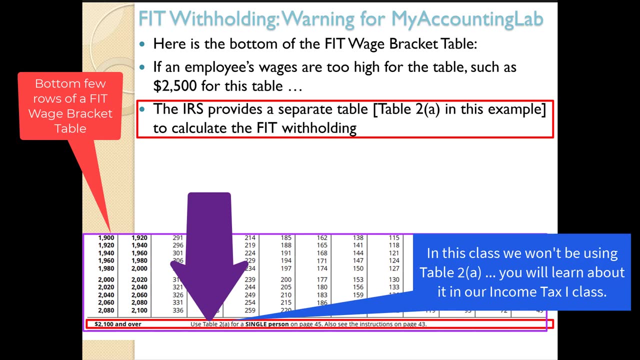 employee's wages are too high for this table, such as $2,500. notice, the IRS provides a separate table in this example to calculate the federal income tax withholding. okay, so no problem, if it goes off the table, then you just go to table to a and this shows you how to do the calculation for it. but in 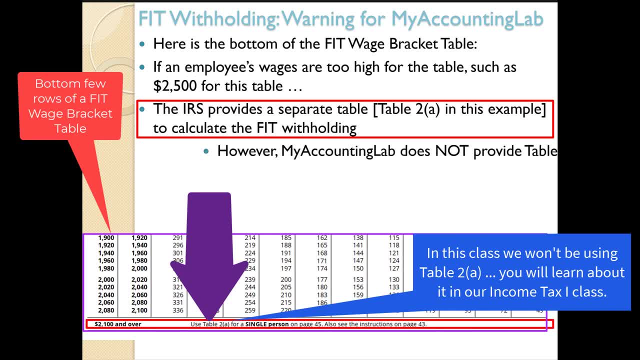 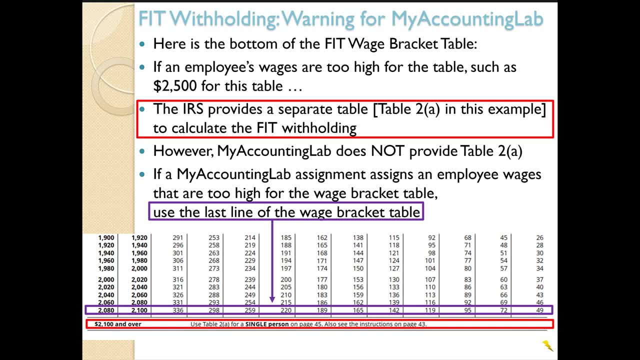 my accounting lab there is no table to a. so if I'm I accounting lab assignment assigns an employee wages that are too high for the wage bracket table, such as $2500 in this table, then just use the last line of the wage bracket table. hopefully, my accounting 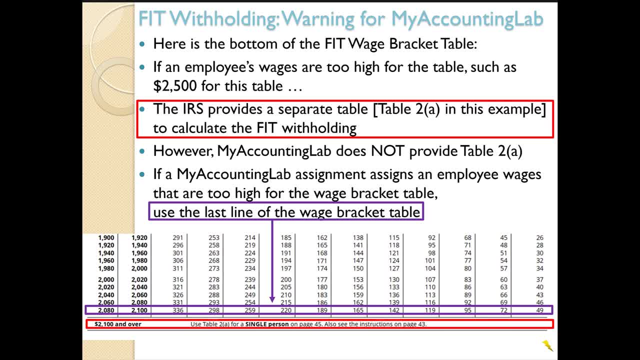 level will fix that problem and it's rare that this problem happens. but remember, on the random problems they might, on the problems with random numbers, they might randomly give you a number that does not fit on the table. it's too big. so in that case, for my accounting lab, just use that last row. 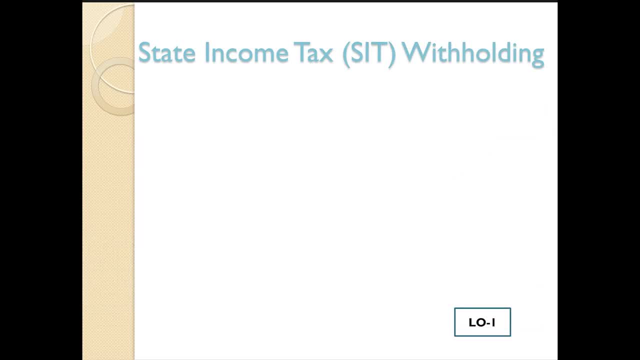 now some states have todo there, some states don't have todo and they do not have total. so we say: a sit a state income tax and you will have to withhold for that. each state has its own state tax laws. most states charge a state income tax, but at this.